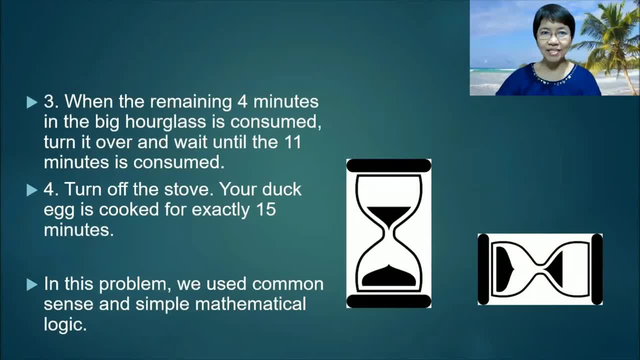 4 minutes in the big hourglass is consumed, turn it over and wait until the 11 minutes is consumed. Turn off the stove. Your duck egg is cooked for exactly 15 minutes. In this problem, we used common sense And simple mathematical logic. Let us define logic. 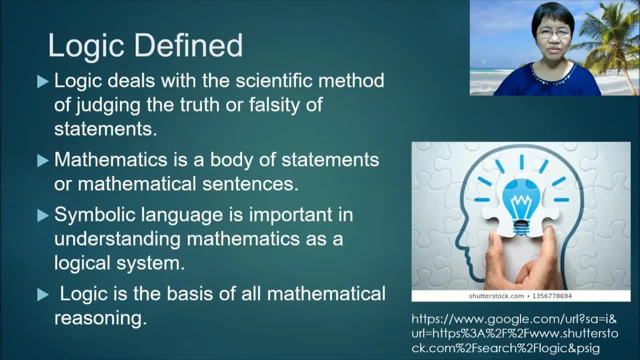 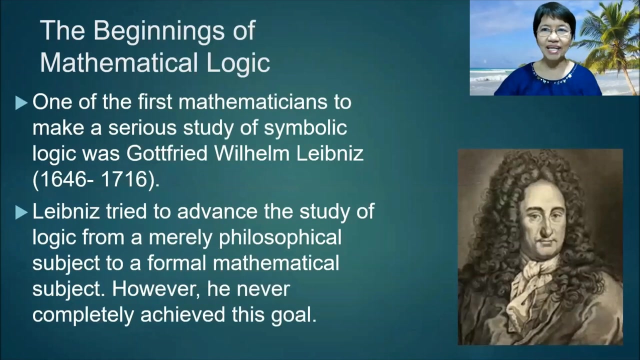 Logic deals with a scientific method of judging the truth or falsity of statements. Mathematics is a body of statements or mathematical sentences. Symbolic language is important in understanding mathematics as a logical system. Logic is the basis of all mathematical reasoning. Let us now trace the beginnings of mathematical logic. 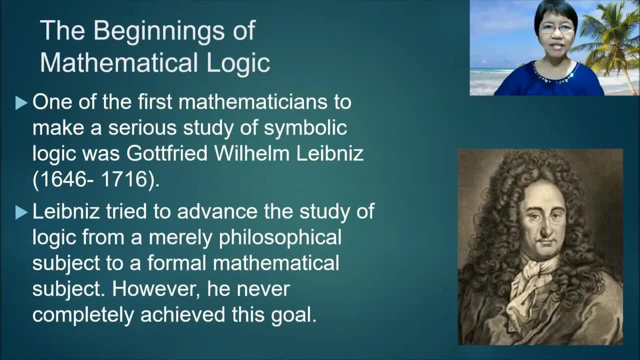 One of the first mathematicians to make a serious study of symbolic logic was Gottfried Wilhelm Leibniz. Leibniz tried to advance the study of logic from a merely philosophical subject to a formal, a mathematical subject. However, he never completely achieved this goal. Many years later, several mathematicians showed evidence that logic works just like reason and that representation changes upon it. Many years later, several maniacs and mathematicians in the wahrscheinlich contexts assumed that logic is a system of actorization, and how it is. Nueblets are here to help give chance to a strategic understanding of logic. 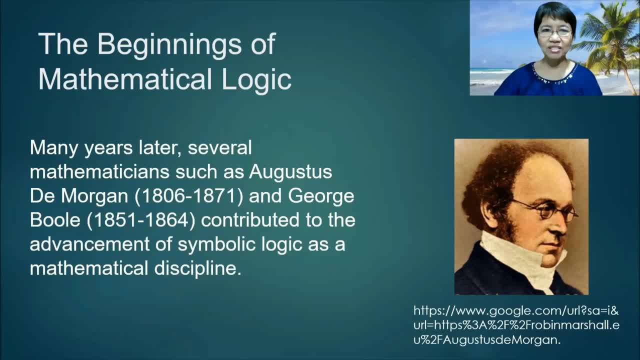 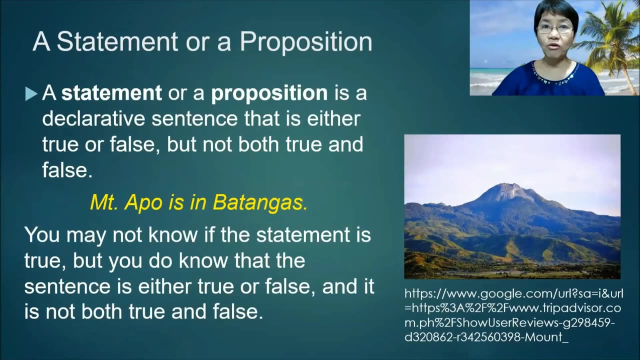 Later, several mathematicians such as Augustus de Morgan and George Boole, contributed to the advancement of symbolic logic as a mathematical discipline. A statement or a proposition- This is a very basic term in logic. A statement or a proposition is a declarative sentence that is either true or false. 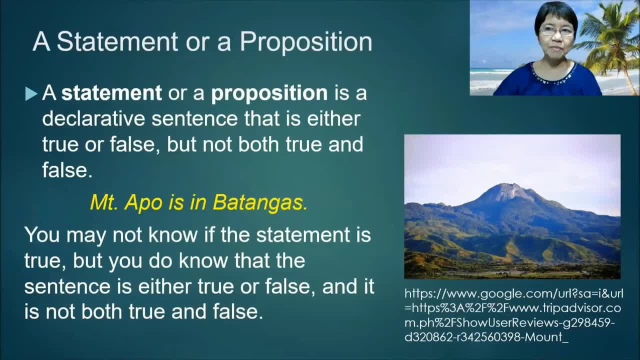 But not both true and false. Example: Mount Apo is in Batangas. You may not know if the statement is true, but you do know that the sentence is either true or false. And it is not both true or false. But the fact is Mount Apo is not in Batangas, but it is in Davao. 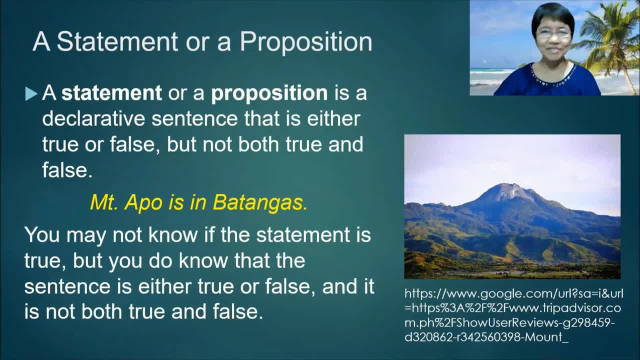 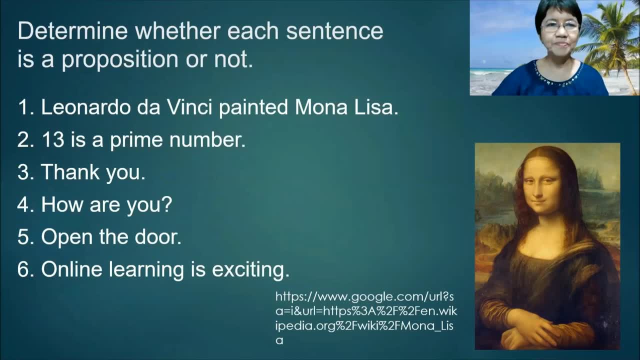 So this sentence is false. Yes, Determine whether each sentence is a proposition or not. Number one: Leonardo da Vinci painted Mona Lisa. This is a true statement, and it is a proposition. Number two: thirteen is a prime number- Another true statement. 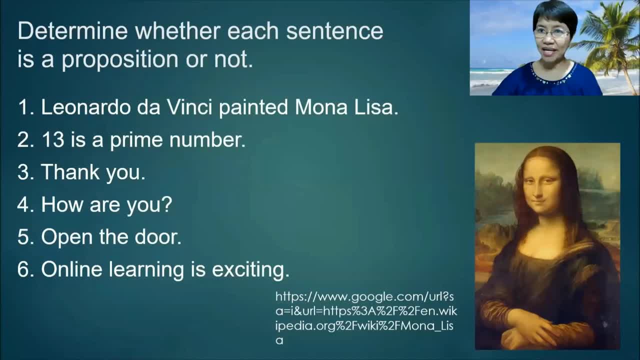 Another proposition. Number three: thank you. Thank you is an expression of gratitude, but you cannot say whether it's true or false, So this is not a proposition. And number four: how are you? How are you is a question. 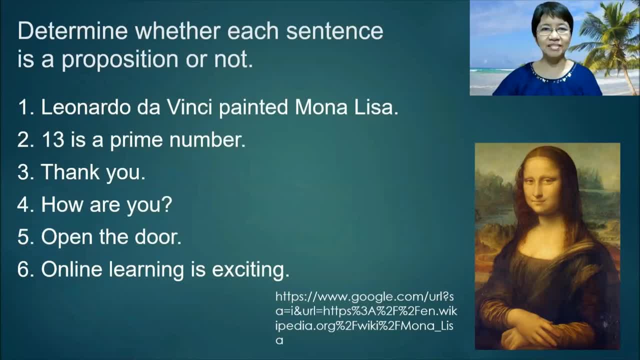 And it is not a proposition. It is not a declarative sentence. Number five: open the door. It is a command and you cannot say that the command is true or false, So it is not a proposition. The number six: online learning is exciting. 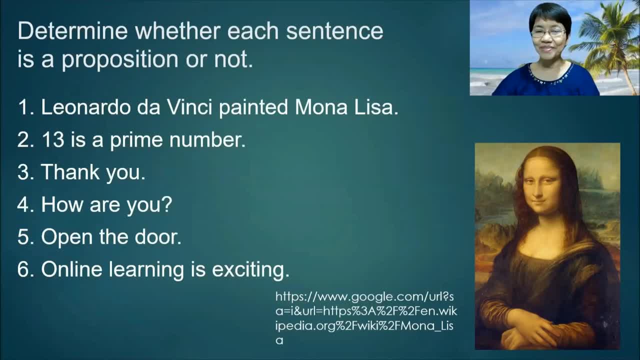 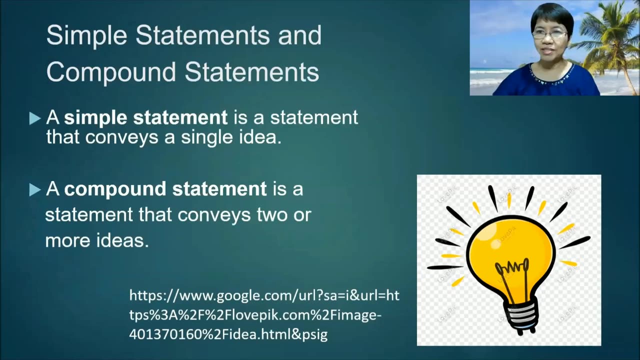 It depends upon the person who is talking. So you can say whether it's true or false depending upon the person who is talking. So this is a proposition: Simple statements and compound statements. A simple statement is a statement that conveys a single idea. 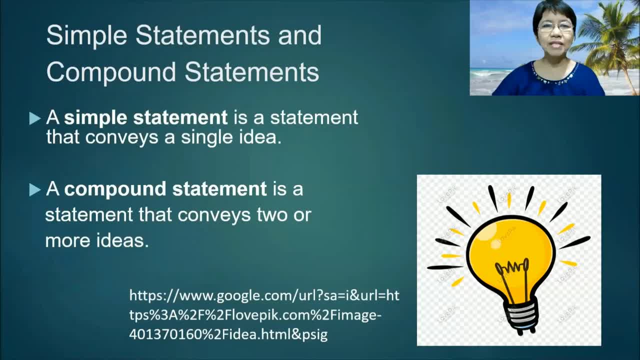 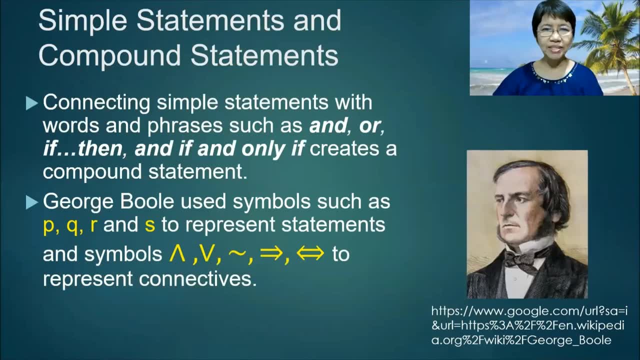 A compound statement is a statement that conveys two or more ideas. Connecting simple statements with words and phrases such as and, or if, then and even only if, creates a compound statement. George Bull used symbols such as P, Q, R and S to represent statements. 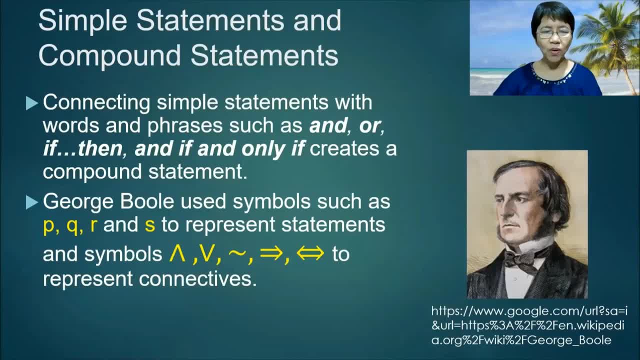 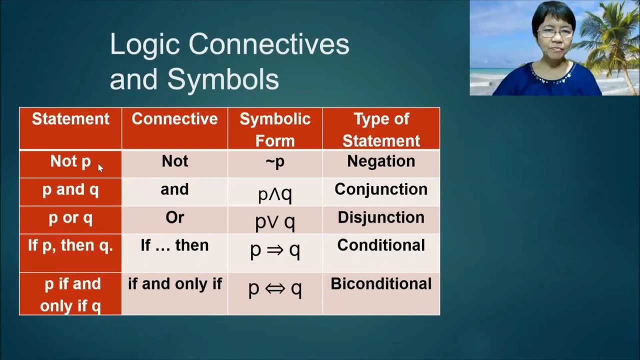 symbols like and or tilde or not, and implication and double implication to represent connectives. here are the logic connectives and symbols. statement not P is a negation and the symbolic form is tilde P or tilde before the P or not P. then we have P and Q. the symbol here is P and then an inverted V and then Q, so P. 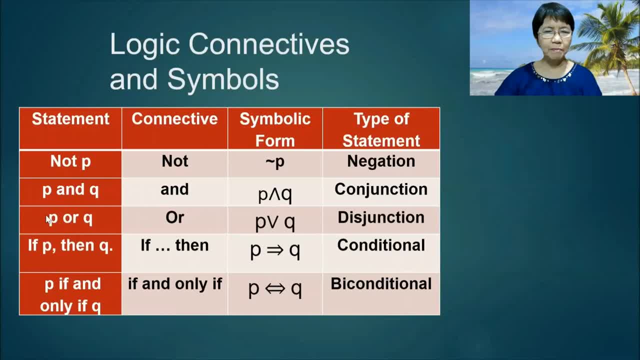 and Q. this is a conjunction. P or Q is a disjunction and the symbol is P, and then we have a letter V and that is P or Q and P. if P, then Q is a conditional and P if, and only if, Q is a biconditional and the 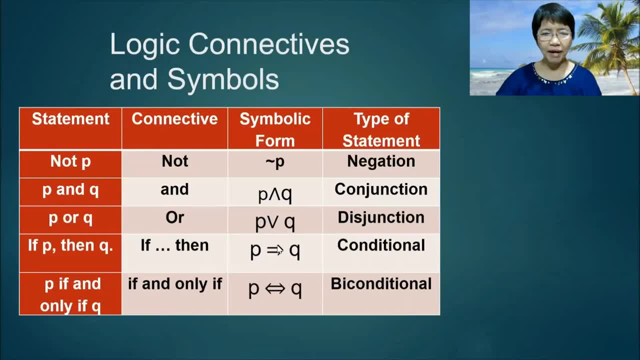 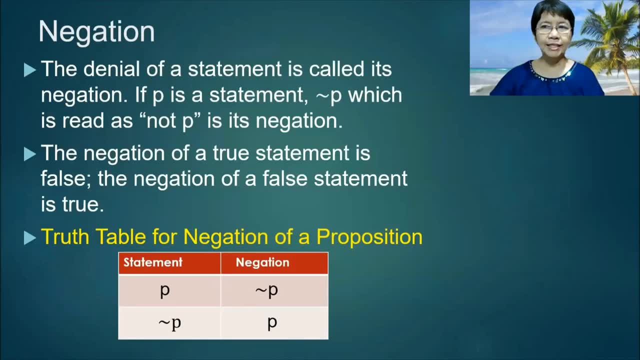 symbols are a one-way arrow and a two-way arrow for the biconditional negation. the denial of a statement is called its negation. if P is a statement, not P, which is read as not P is negation, is its negation. the negation of a true statement is false and the negation of a 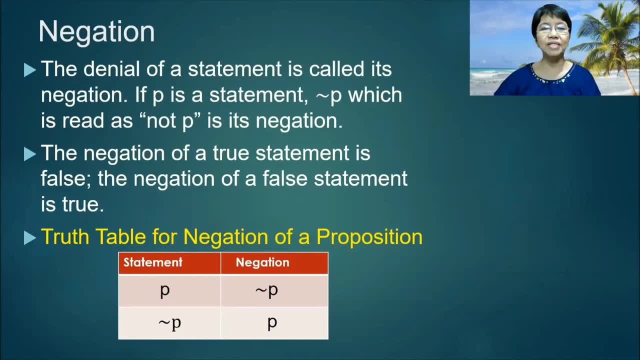 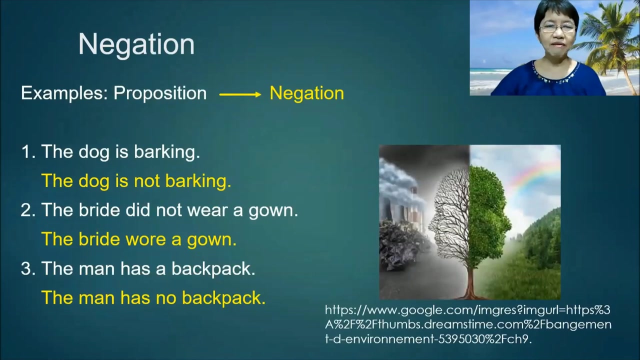 false statement is true. here is the truth table for negation of a proposition. so if the statement is P, the negation is not P, and if the statement is stated in the negative or not P, then its negation is positive or P. examples of negation: from a proposition to a negation, number one: the dog is 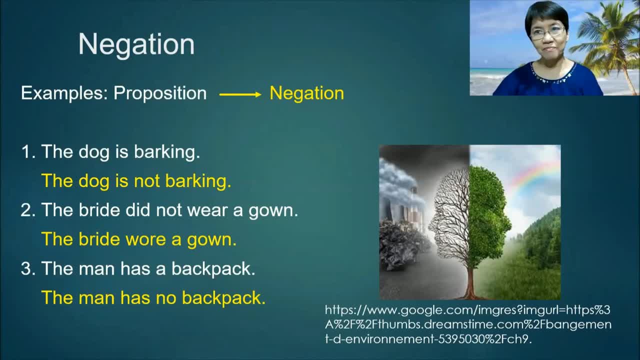 barking. the negation is: the dog is not barking. number two: the bride did not wear a gown, so the negation is: you just remove the words, did not? the bride wore a gown? and number three: the man has a backpack. the negation is a. 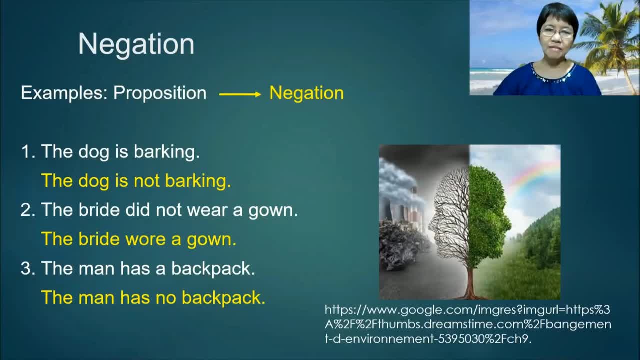 backpack. here are examples in case you fall asleep or if you say something wrong, the man has no backpack. look at the picture here. the the half of the picture is a negation of the other half, so the left side of the picture is gloomy, dry and dead and 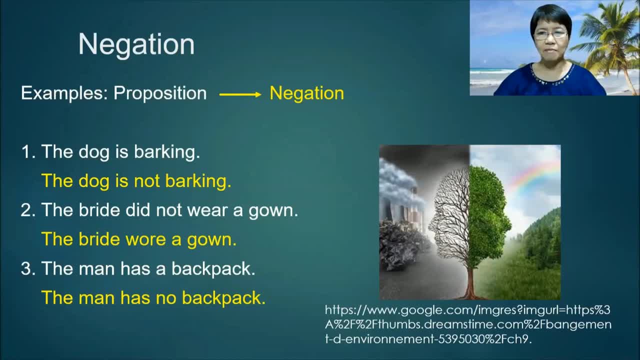 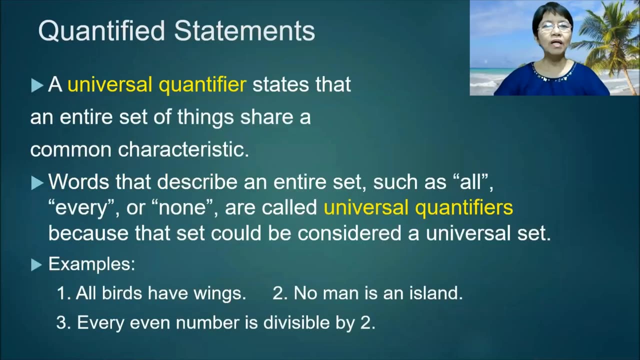 the right half of the picture is bright, alive and green, so they are exact opposites and they are negations of one another. quantified statements. a universal quantifier states that an entire set of things share a common characteristic. words that describe an entire set, such as: 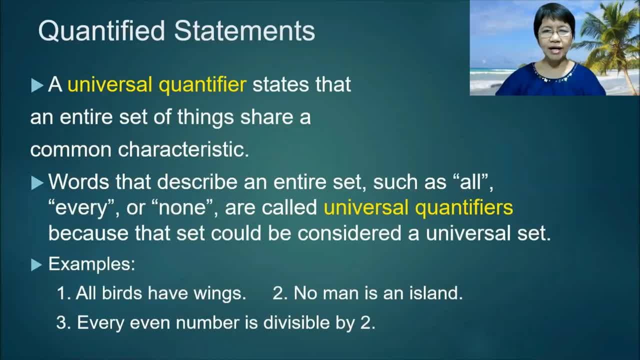 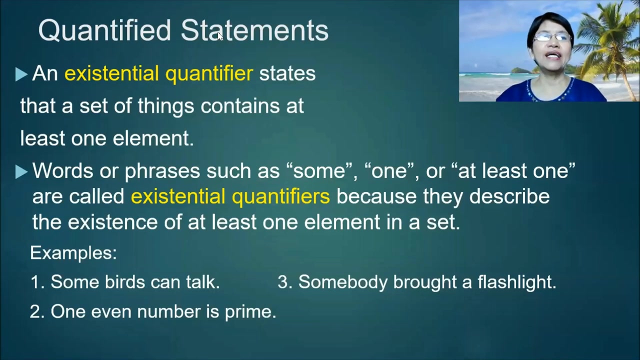 all, every or none are called universal quantifiers because the set could be considered a universal set. examples: all birds have wings. number two: no man is an island. and number three: every even number is divisible by two. an existential quantifier. quantifier states that a set of things contains at least one element, words or 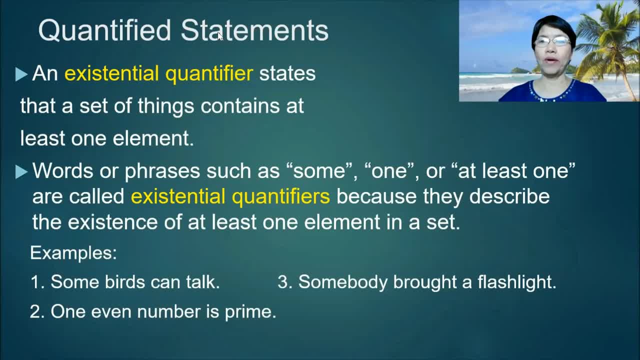 phrases such as some one or at least one are called existential quantifiers because they describe the existence of at least one element in a set examples. some birds can talk number two, one even number is prime. number three- somebody brought a flashlight. negations of statements with quantifiers, the word. 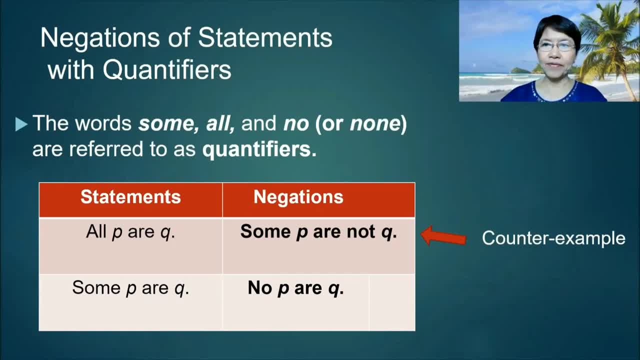 some, all and no or none are referred to as quantifiers. so if the statement is all P are Q, the negation is some P are not Q, or at least you can give one counter example to prove that not all P are Q. and then if the statement is some P are Q, then the negation is no P are Q here. 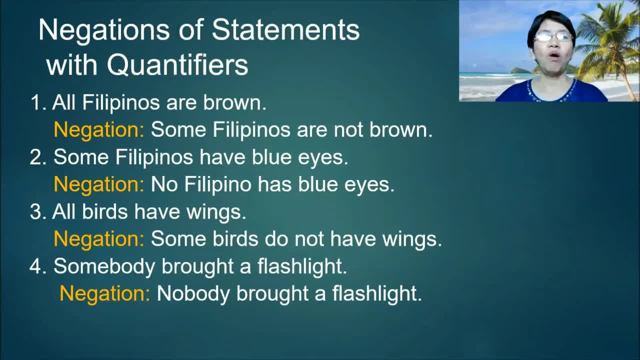 are some examples. number one: all Filipinos are brown- negation. some Filipinos are not brown. number two: some Filipinos have blue eyes- negation. no Filipino has blue eyes. number three: all birds have wings- negation. some birds do not have wings. and number four: somebody brought a flashlight- negation. nobody brought a. 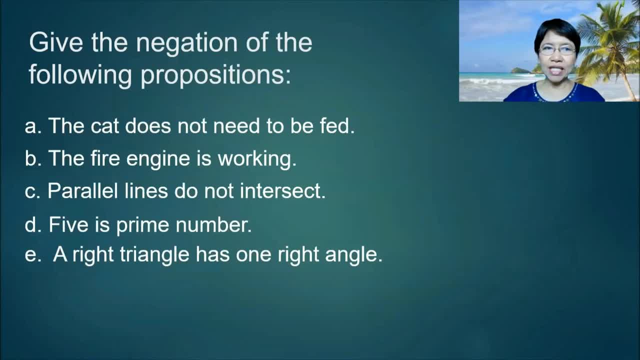 flashlight give the negation of the following propositions: the cat does not need to be fed. the cat needs to be fed. B- the fire engine is working- negation. the fire engine is not working. see: parallel lines: do not intersect. negation. parallel lines intersect. D. 5 is a prime number. negation. 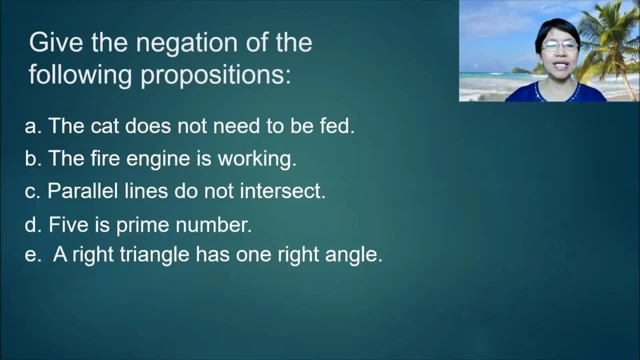 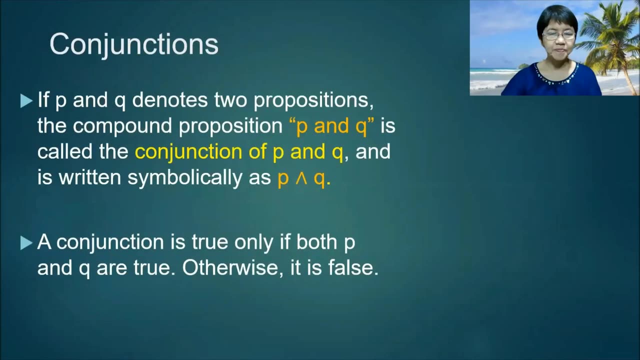 5 is not a prime number. e: a right triangle has one right angle and the negation is a right triangle does not have one right angle. conjunctions: if P and Q denote two propositions, the compound proposition P and Q is called the conjunction of P and Q and is written symbolically as P and Q a. 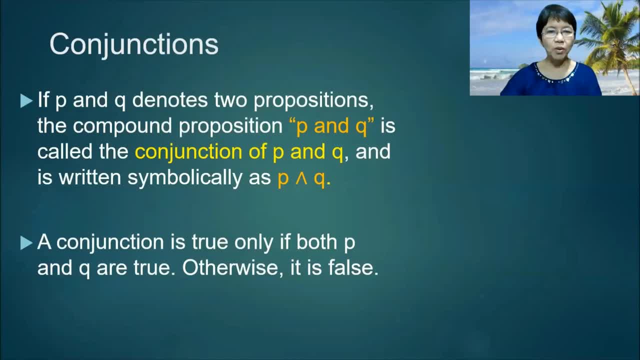 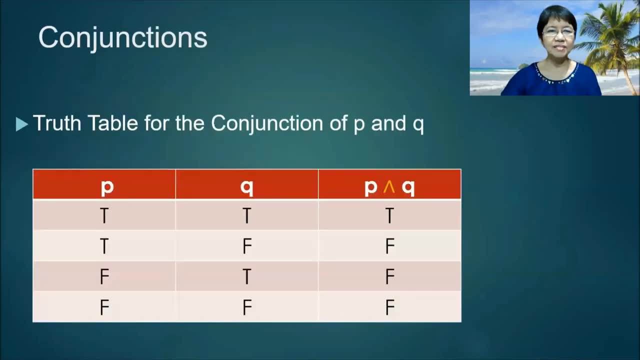 conjunction is true only if both the right and left angles are not connected. P and Q are true, otherwise it is false. here is the truth. table for the conjunction of P and Q. suppose P and Q are both true, then P and Q is true. but if either P or Q is false, then the conjunction is false, or? Or if both P and Q are false, then the conjunction is also false. So there is only one condition for the conjunction to be true, And this is if both P and Q are true. Examples Determine the truth value of the following conjunctions: 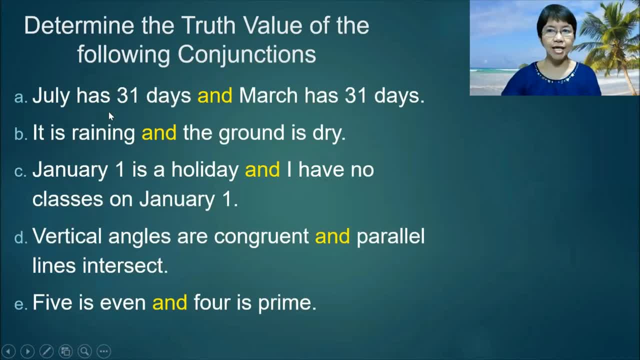 So July has 31 days and March has 31 days. So July has 31 days, That's true, March has also 31 days. So if you get the conjunction of the two, true plus true, equals true Letter B. 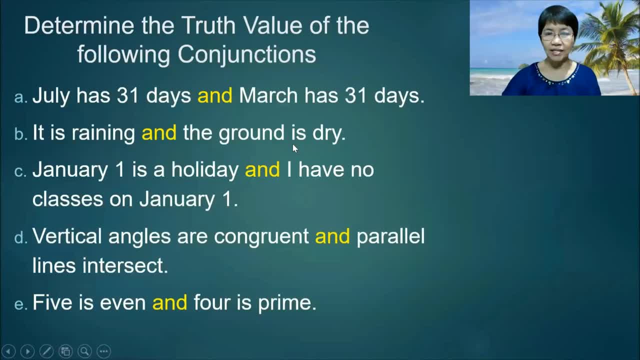 It is raining and the ground is dry. So if the first statement is true, the second statement is also true. The third statement cannot be true. So this is a false conjunction And letter C. January 1 is a holiday and I have no classes on January 1.. 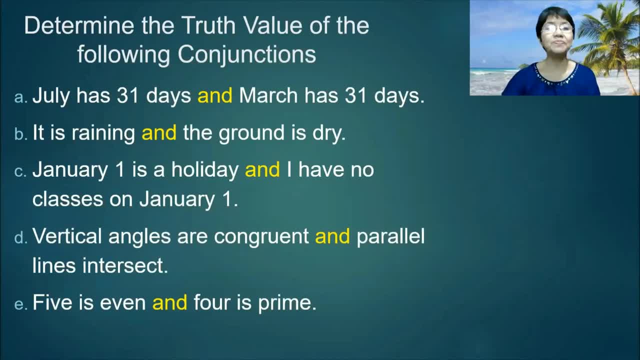 So both are true and the conjunction is true. Letter D: Vertical angles are congruent and parallel lines intersect, So the first is correct, but the second is false. So the second statement is wrong. So the conjunction is wrong or false. 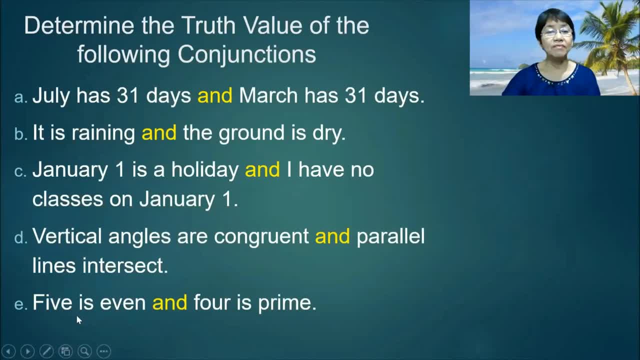 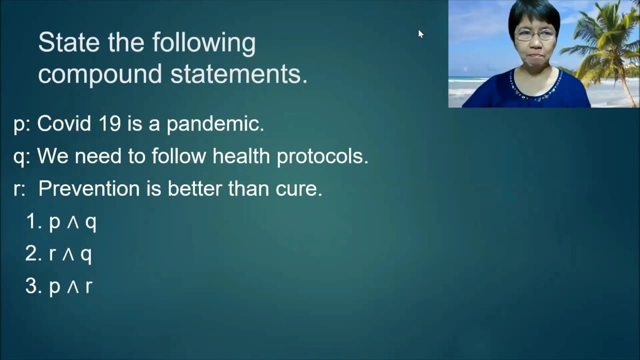 Letter E, 5 is even and 4 is prime, So they are both false. So the conjunction is false. So the conjunction is false. So the conjunction is false. State the following compound statements: P COVID-19 is a pandemic. 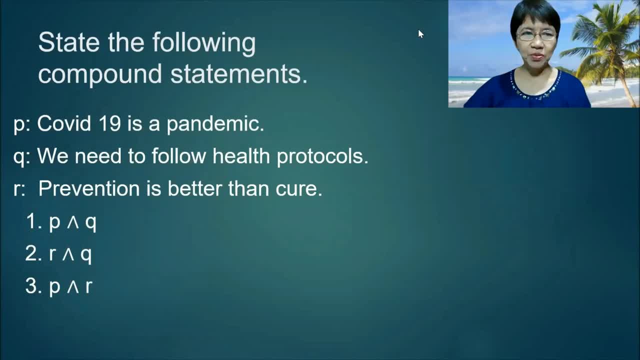 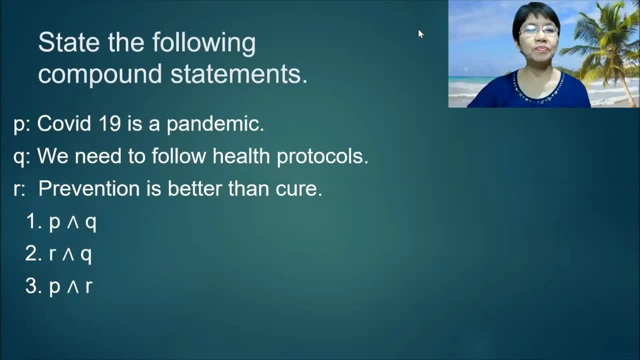 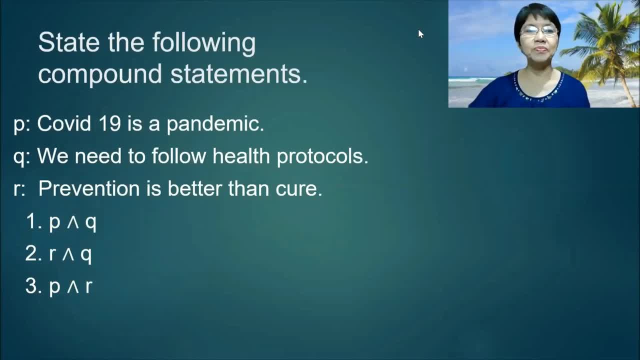 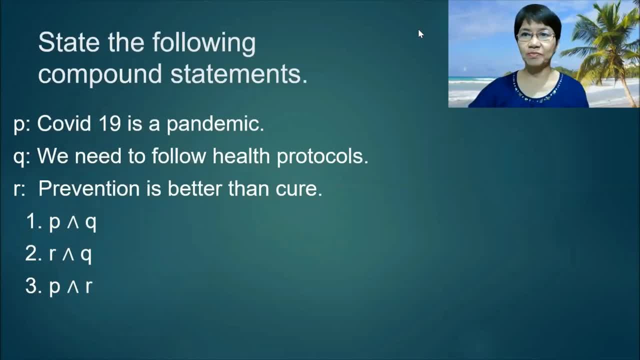 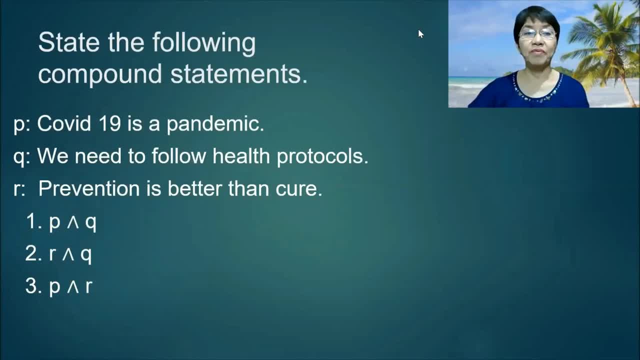 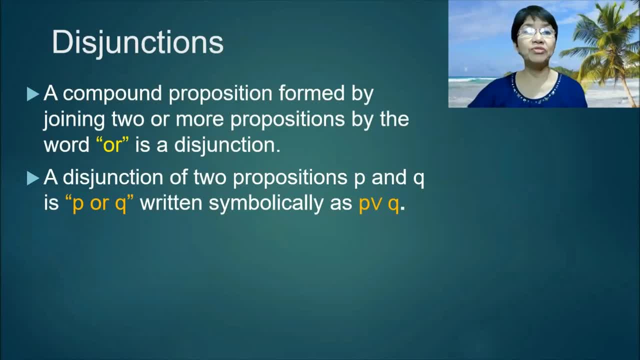 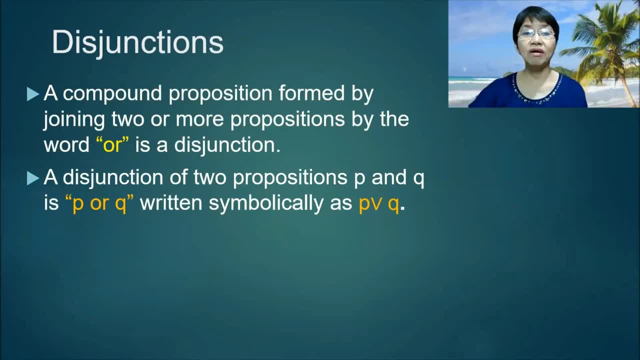 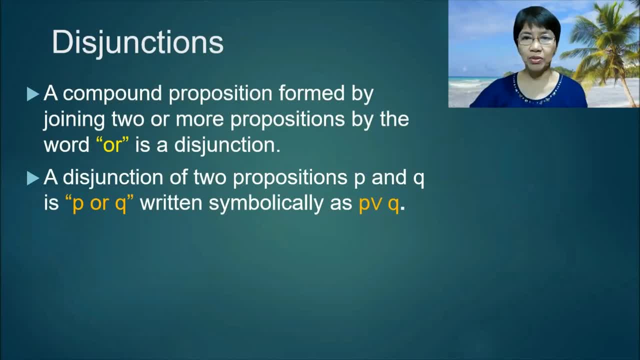 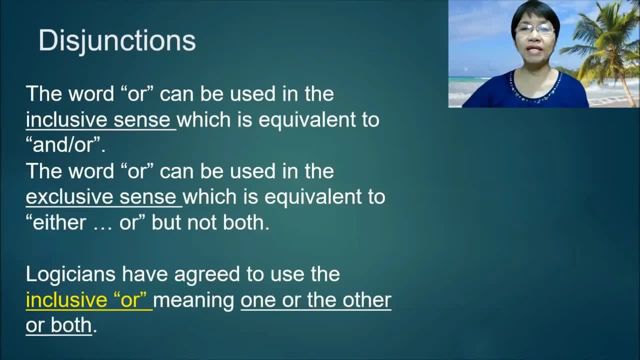 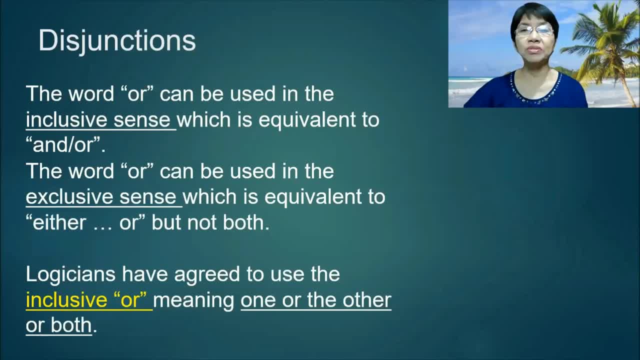 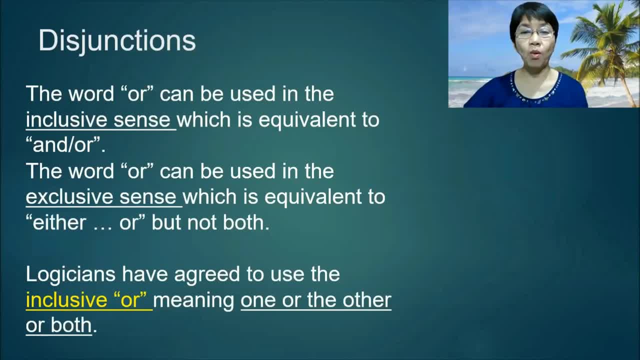 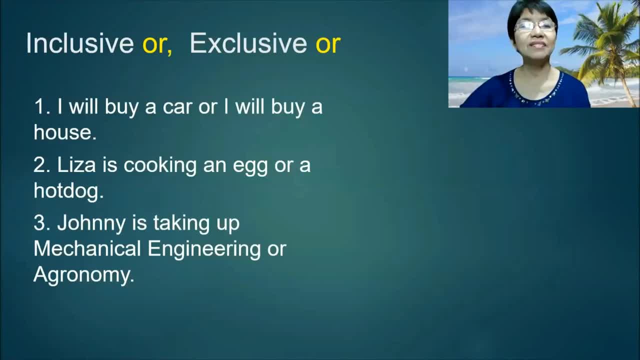 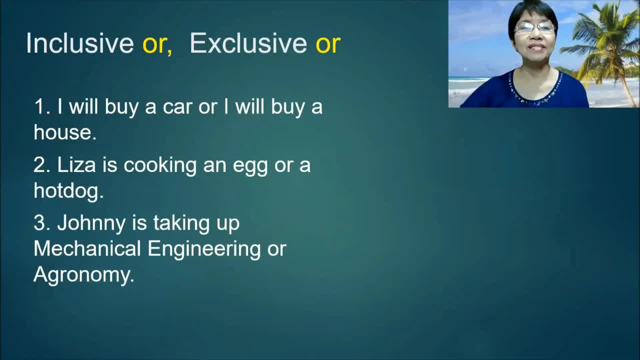 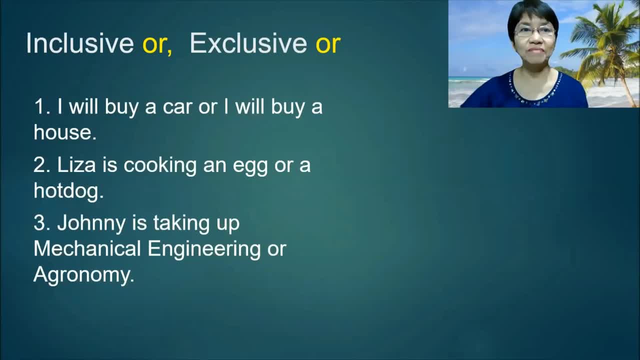 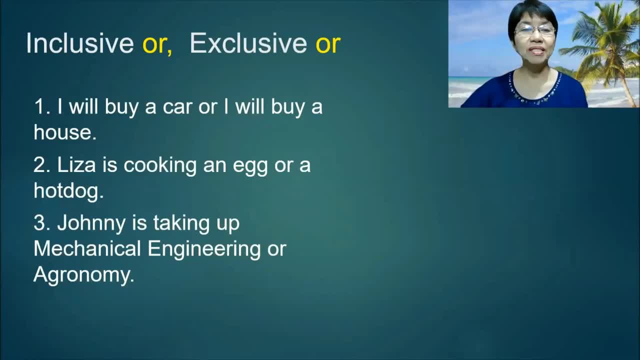 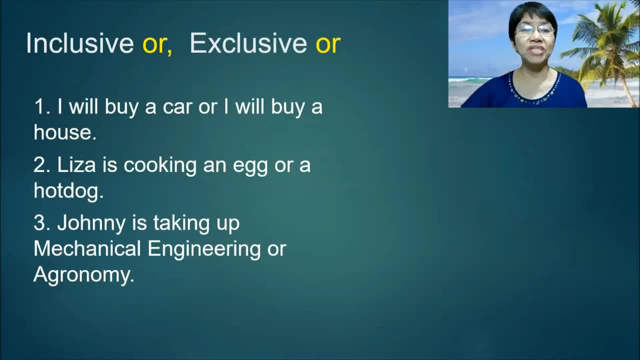 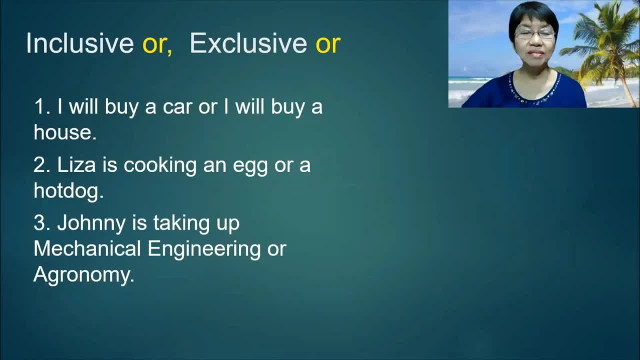 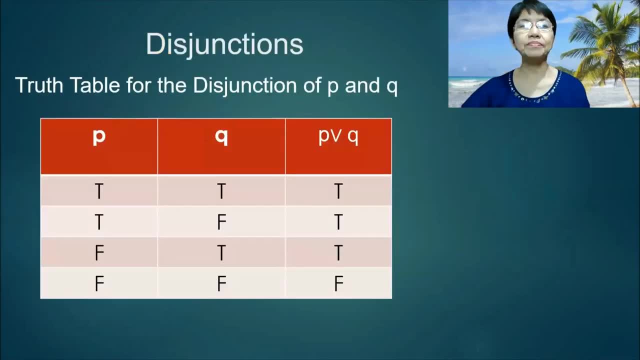 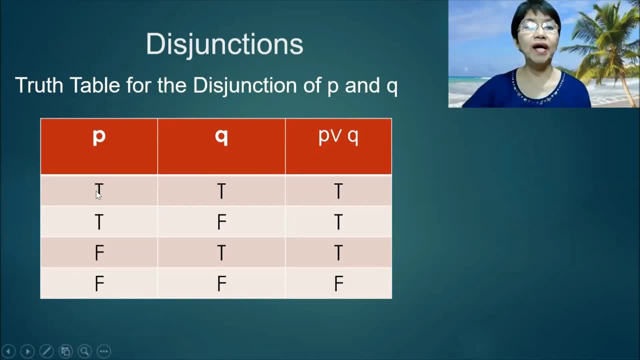 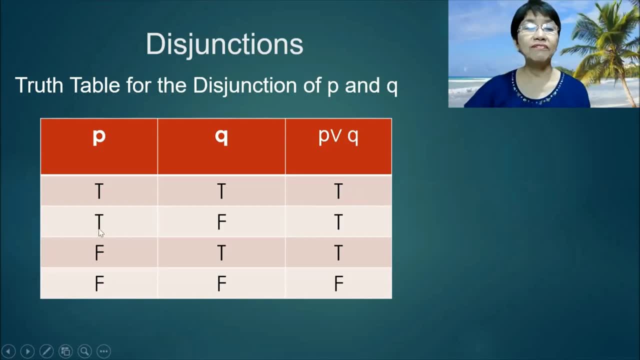 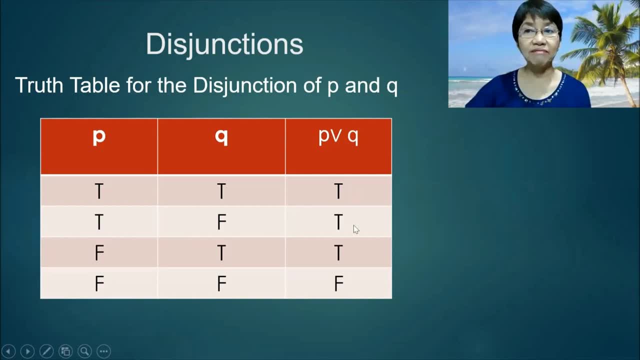 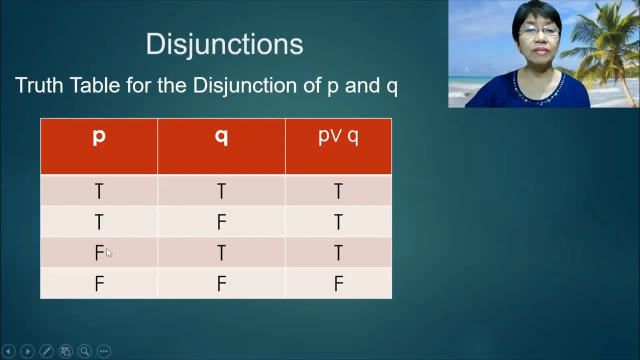 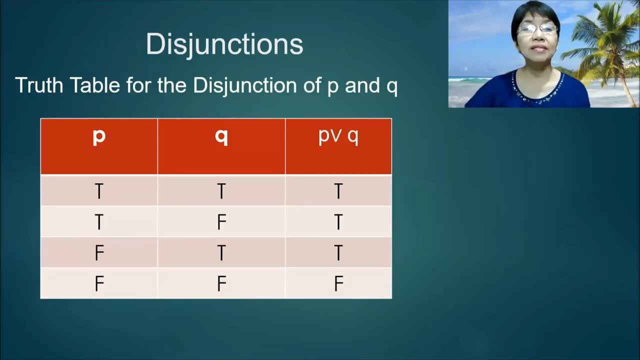 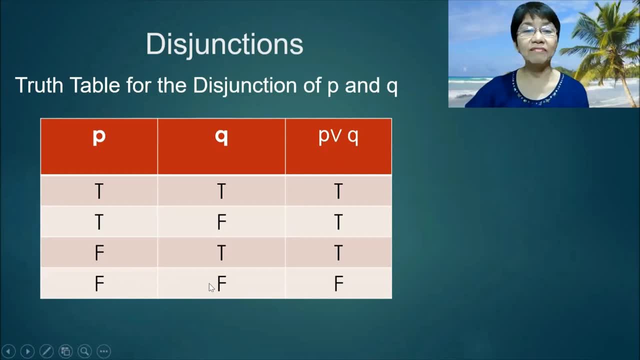 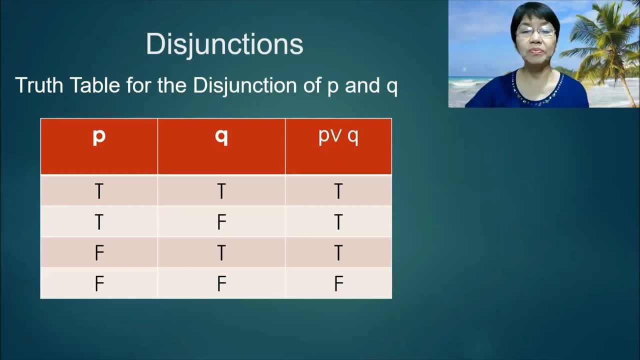 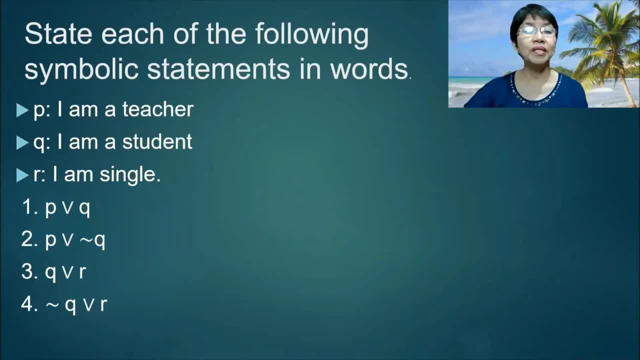 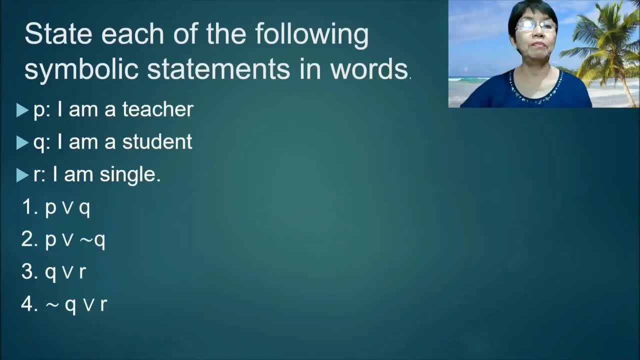 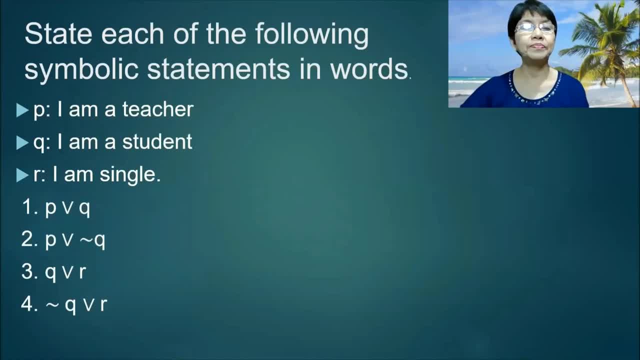 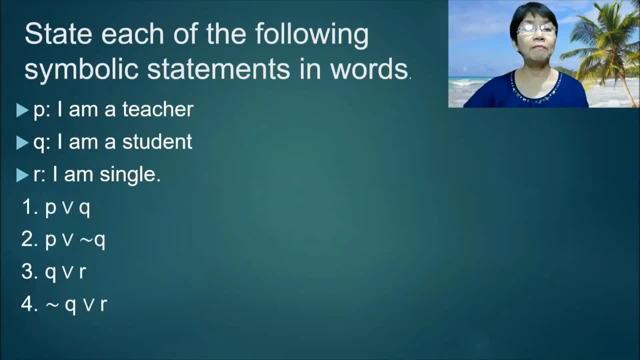 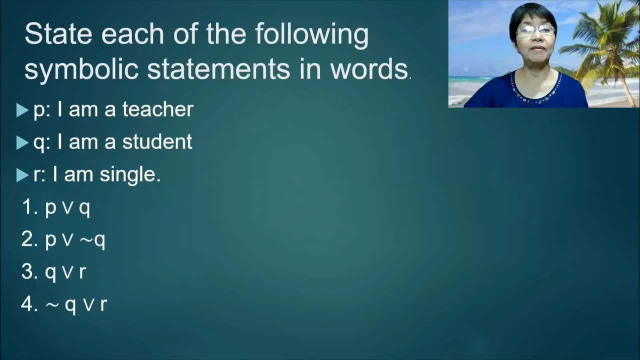 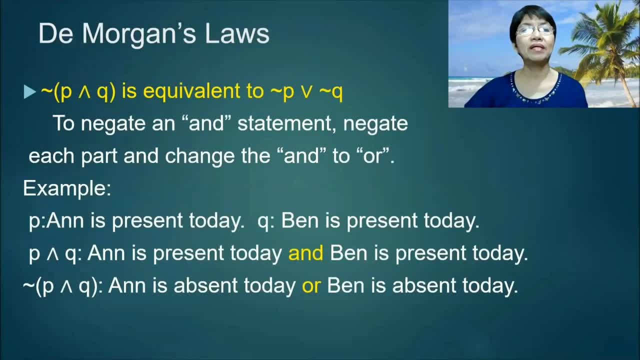 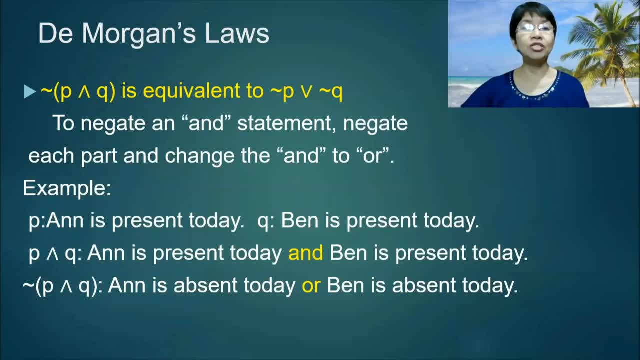 To negate an AND statement, negate each part and change the AND to OR. examples: If P is AND is present today and Q is, BAN is present today, P and Q is AND is present today and BAN is present today, NOT P and Q means AND is absent today or BAN is absent today. 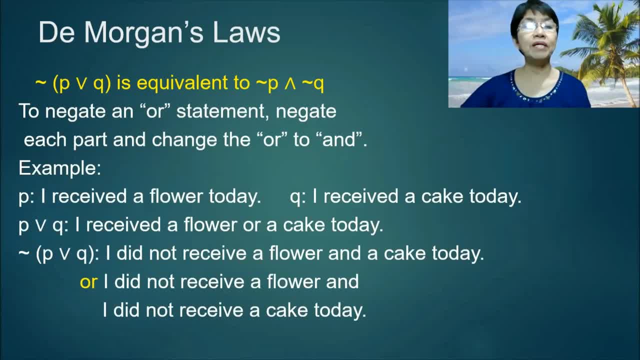 The Morgan's Laws, NOT P or Q is equivalent to NOT P and NOT Q. To negate an OR statement, negate each part and change the OR to AND. Example: P- I received a flower today. Q. I received a cake today. 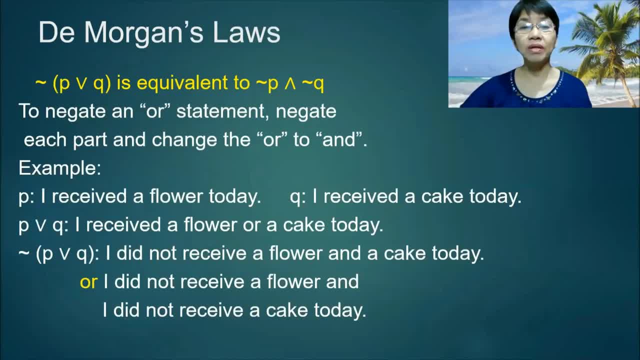 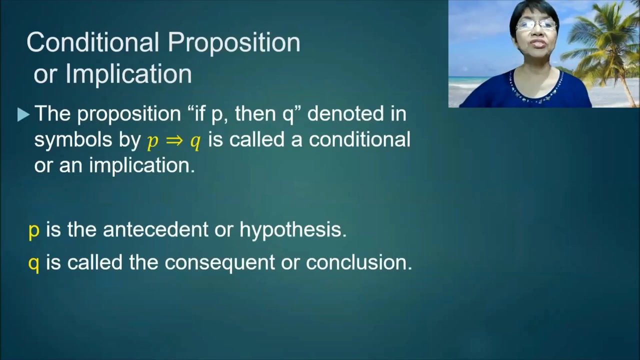 P or Q. I received a flower or a cake today, NOT P or Q. I did not receive a flower and a cake today, OR I did not receive a flower and I did not receive a cake today. Conditional Proposition or Implication. 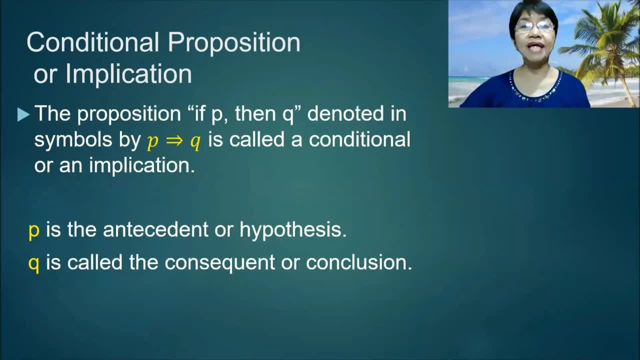 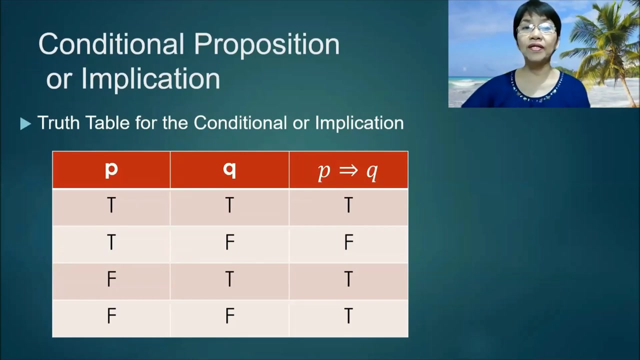 The proposition. if P then Q, denoted in symbols by P, implies Q is called a conditional or an implication, P is the antecedent or the hypothesis AND Q is the consequent or the conclusion. And here is the truth. table for the conditional or implication. 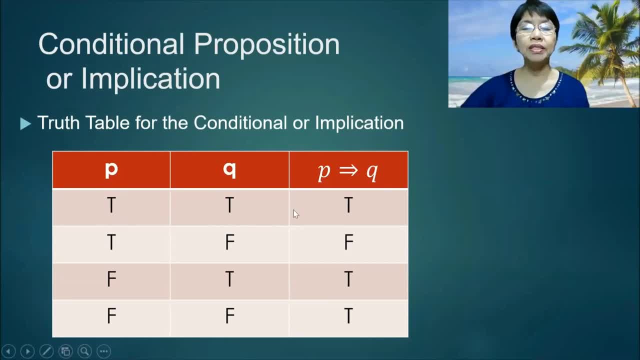 If P is TRUE AND Q is TRUE, the implication P implies Q is TRUE. If P is TRUE AND Q is FALSE, the implication is FALSE. The implication of Q gakal is equals to TRUE. If P is false and Q is true, the implication is still true. 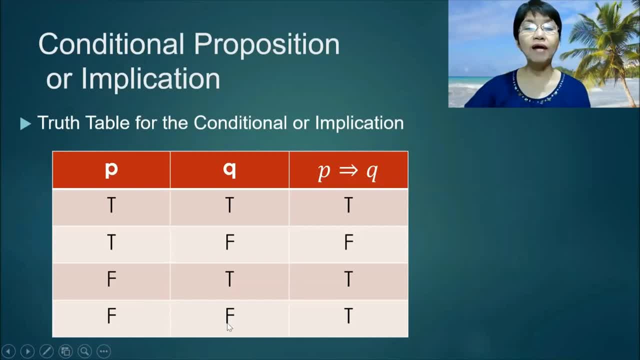 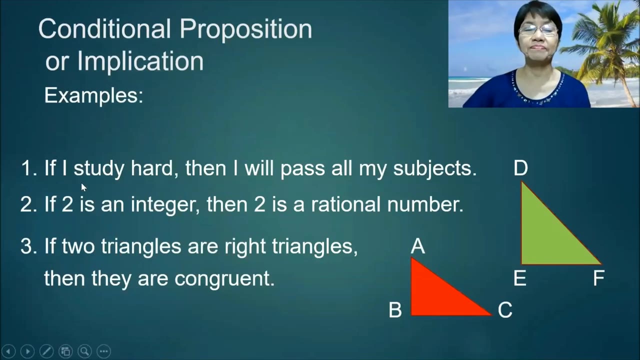 And if both P and Q are false, the implication is true. It's like negative times. negative is positive Conditional proposition or implication. If I study hard then I will pass all my subjects, So it seems logical to believe that both will be true. 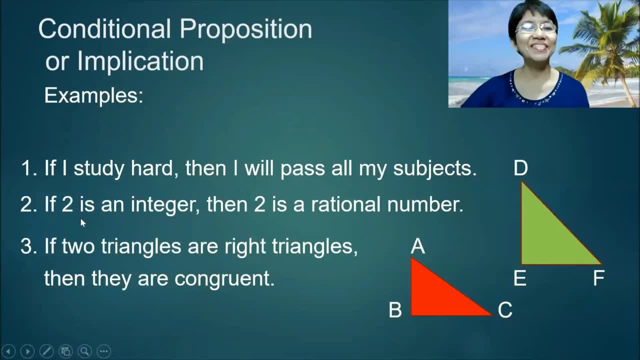 Study hard and pass all your subjects. Number two: If two is an integer, then two is a rational number. The first, or P, is false, True, And two is a rational number, is true. So this is a true implication. Number three: 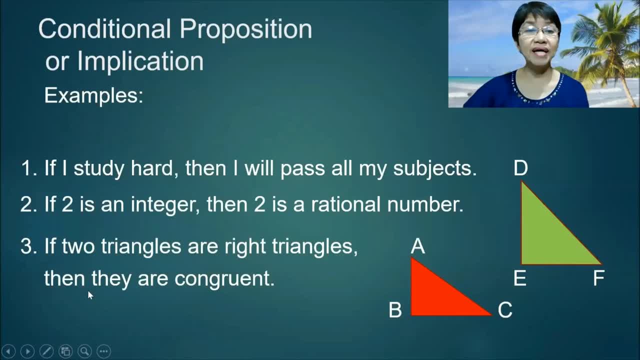 If two triangles are right triangles, then they are congruent. And we have a case here where the two triangles are right triangles, but obviously they are not congruent. So the first statement is true And the second statement is false. So the implication is false. 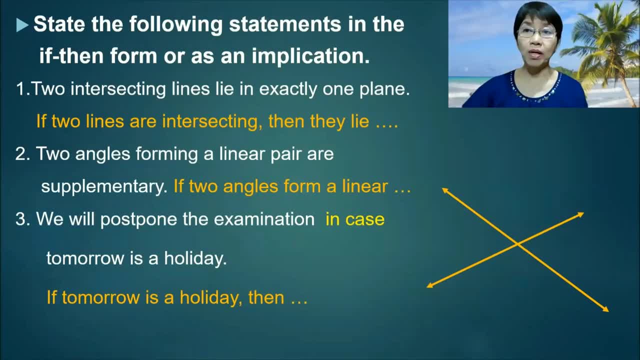 State the following statements in the if-then form or as an implication Number one: Two intersecting lines lie in exactly one plane. So, as an implication, you start with: if So, if two lines are intersecting, then they lie in exactly one plane.